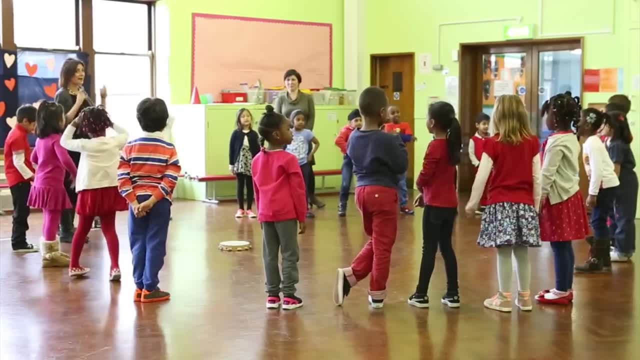 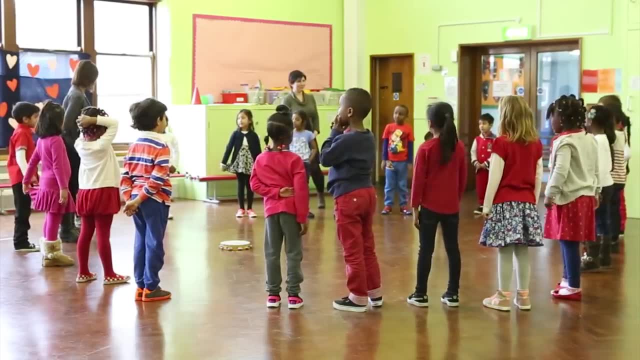 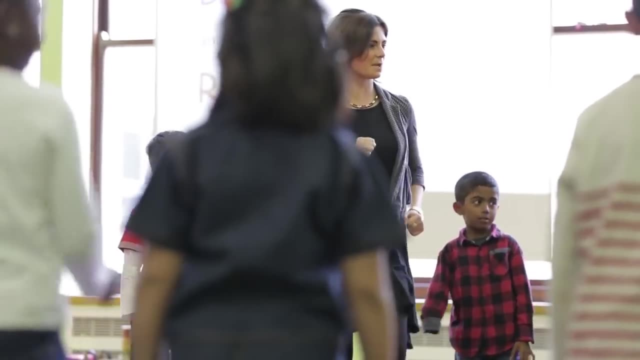 Good morning everybody. Good morning Missy, Good morning everyone. H-E-L-L-O. H-E-L-L-O. This is how we say hello. This is how we say hello. Move your feet to the beat. Move your feet to the beat. 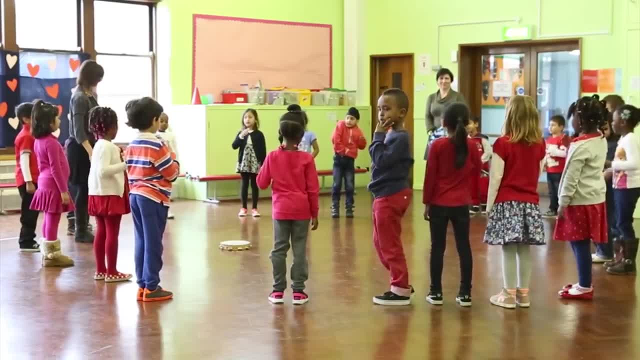 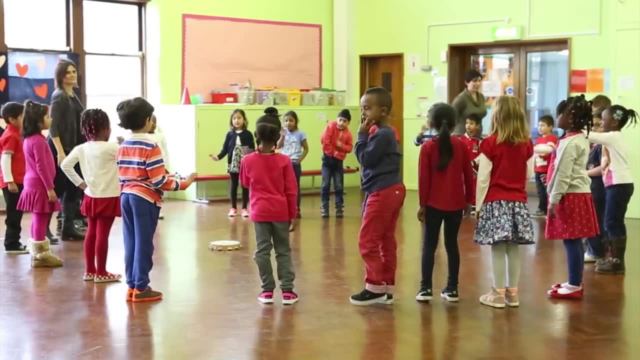 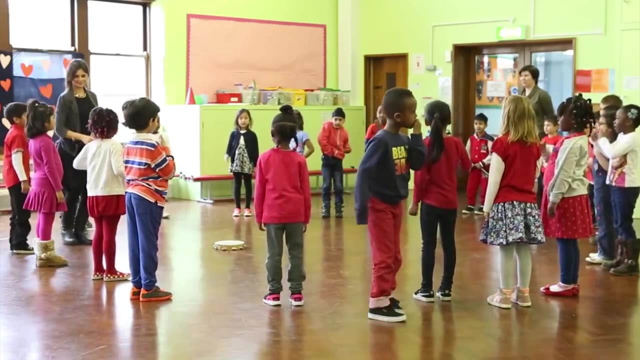 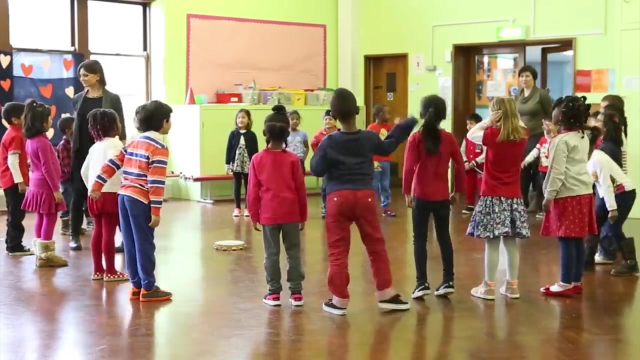 Can you feel my heartbeat? Can you feel my heartbeat? H-E-L-L-O. This is how we say hello. This is how we say hello. Move your feet to the beat. Move your feet to the beat. Can you feel my heartbeat? H-E-L-L-O. H-E-L-L-O. This is how we say hello. This is how we say hello. 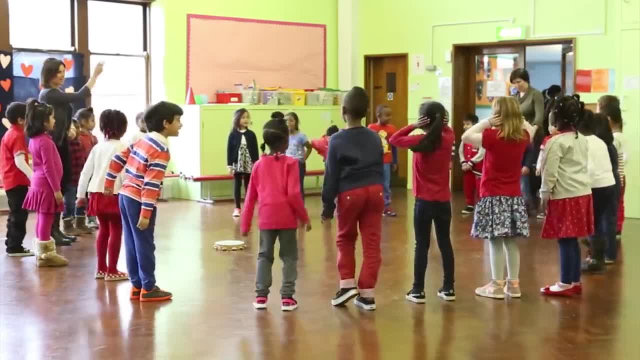 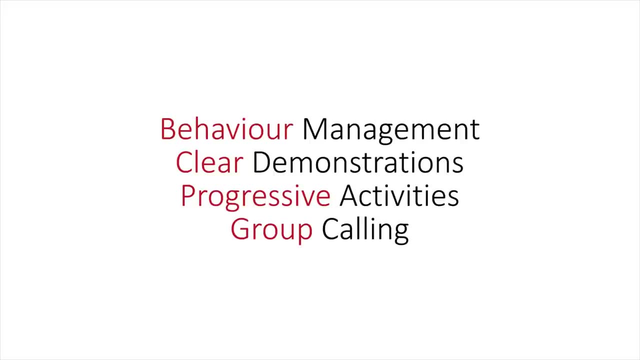 Move your feet to the beat. Move your feet to the beat. Can you feel my heartbeat? H-E-L-L-O, H-E-L-L-O. This is how we say hello. This is how we say hello. Move your feet to the beat. Move your feet to the beat. 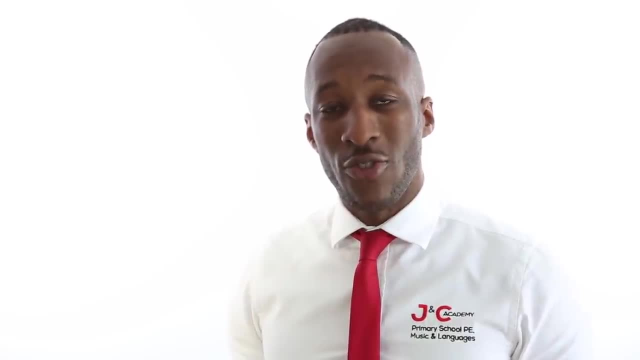 In the main phase of the lesson, the teacher reinforces the expectation for behaviour Before providing a clear demonstration which helps children to improve their performance. Notice how Molly delivers activities which are dynamic and progressive and which clearly link to the main learning objectives. children respond together. helping them to remember key words show me good 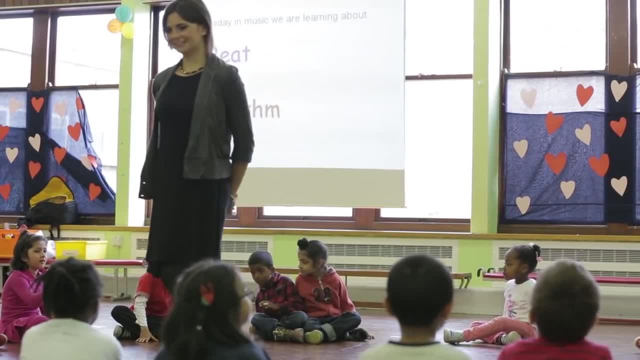 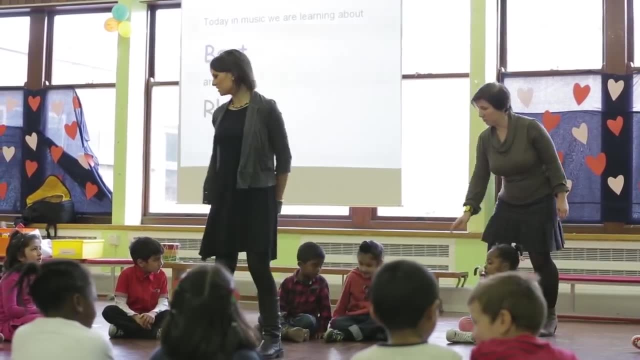 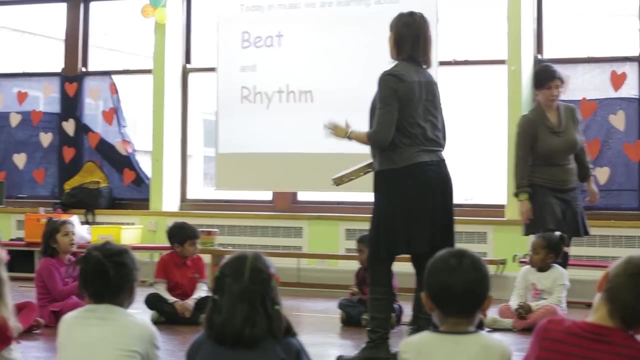 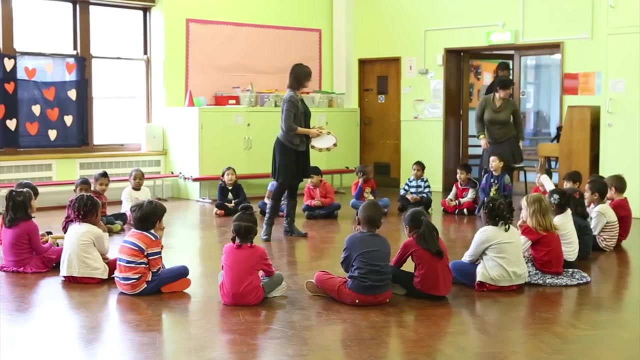 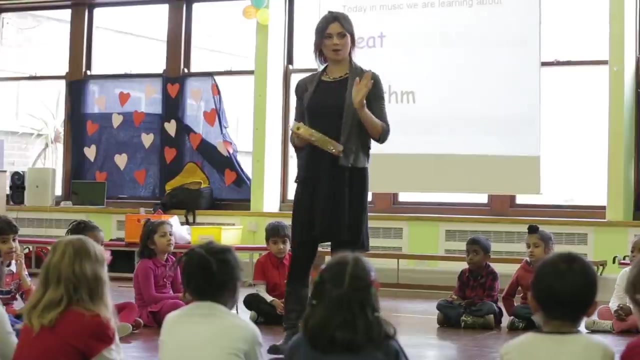 sitting everybody and no talking, so we all know this song. when the music stops, you need to quickly run to the middle of the circle and you need to play the beat. all the rhythm, rhythm. okay, so if we're going, was I tapping the beat or the rhythm somebody? 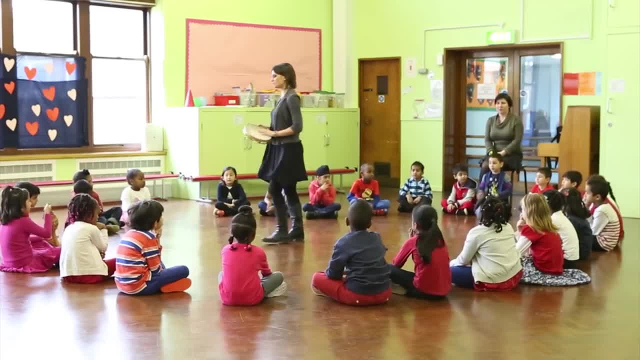 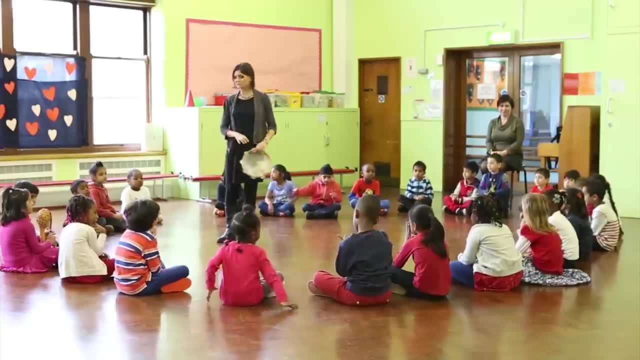 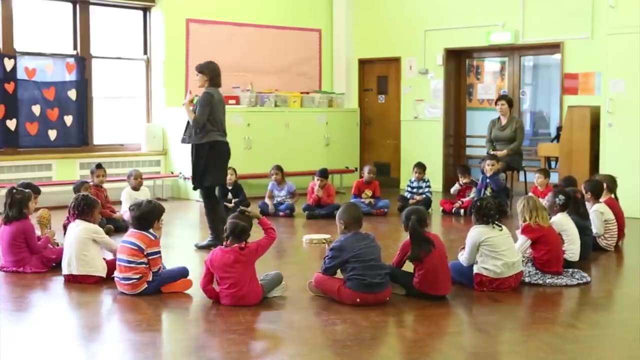 tell me: yeah, I was doing the feet if I was to do this. that is rhythm, fantastic. so if the music stops, you are going to do out of the beat or the rhythm. now I'm going to tell you which one to do. okay, so I want to see if 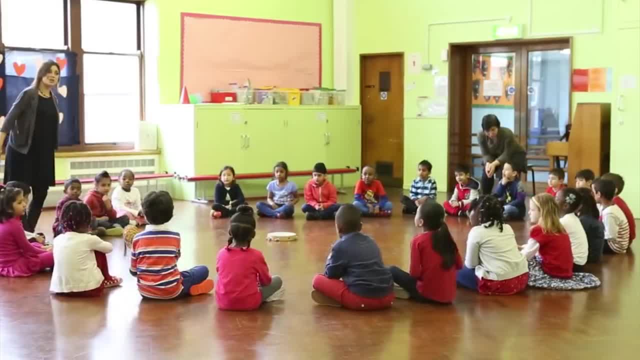 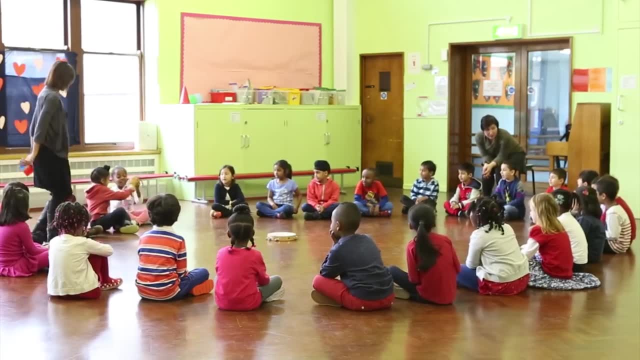 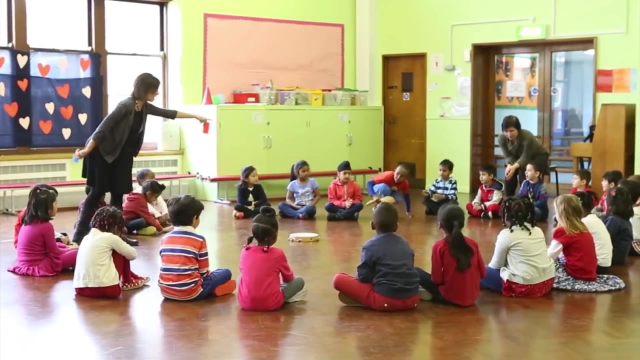 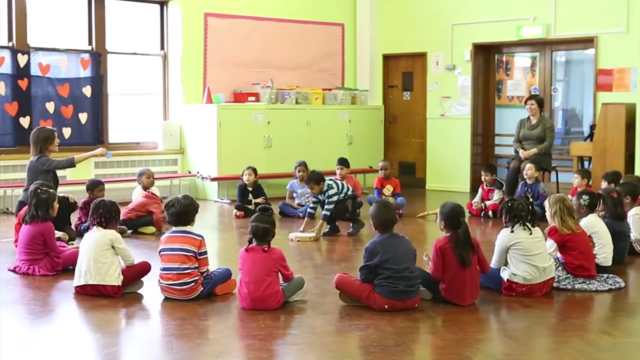 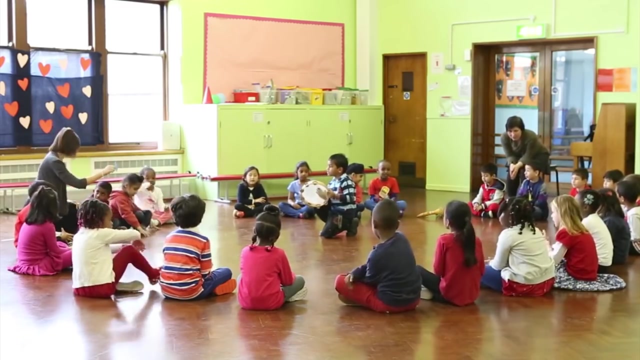 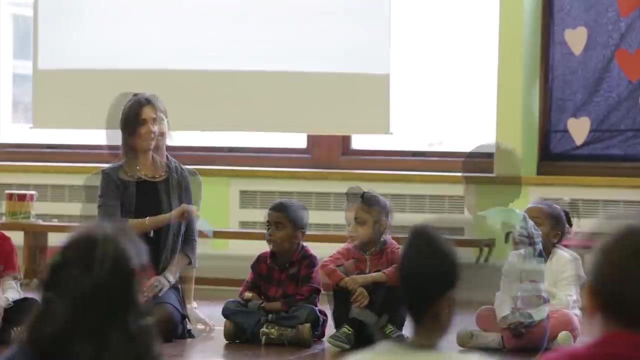 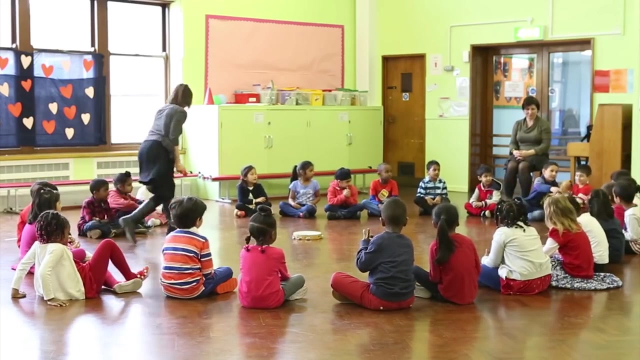 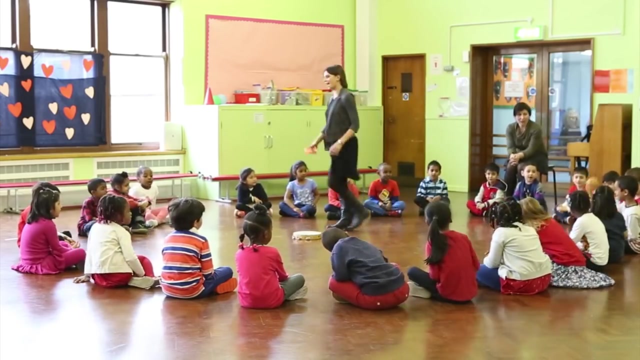 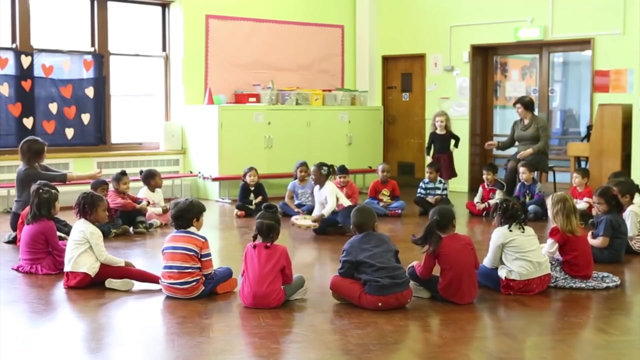 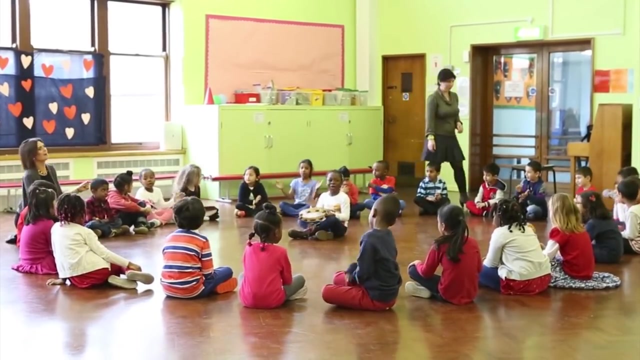 you can do the difference between beat and rhythm. it didn't stop, did it quickly. that's your favourite. Ok, ready, pass it on. Choose an instrument you can play. sing what was on your favourite. Let's see this one. You can play the tambourine- tambourine. 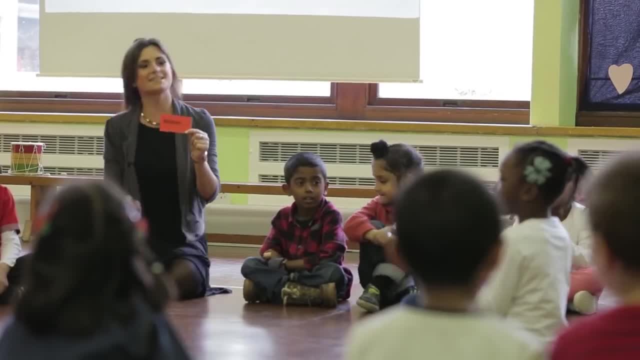 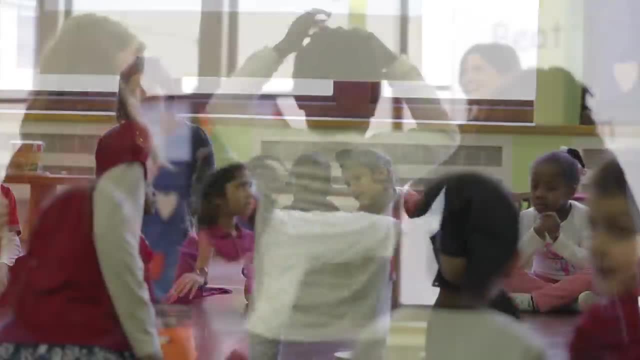 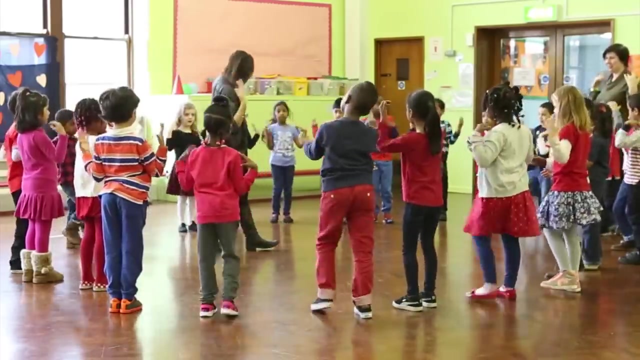 tambourine. you can play the tambourine that's your favourite. Well done, Sing Che che culleye, che che culleye, che che come a karate, che che come a karate, come a. 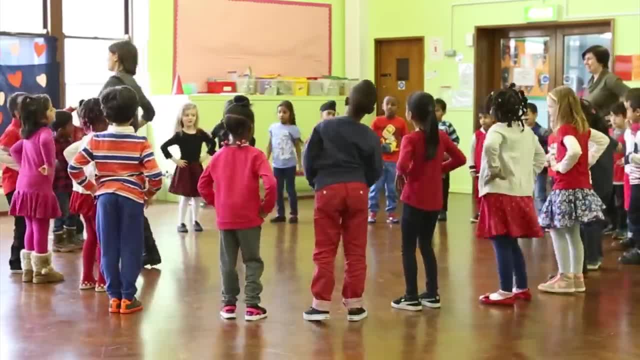 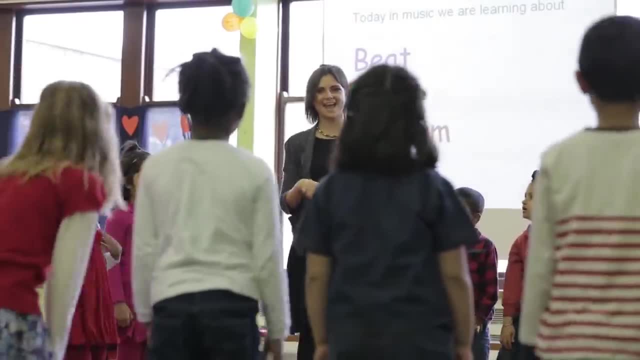 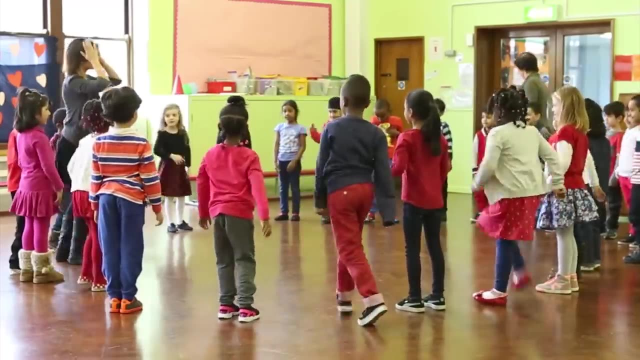 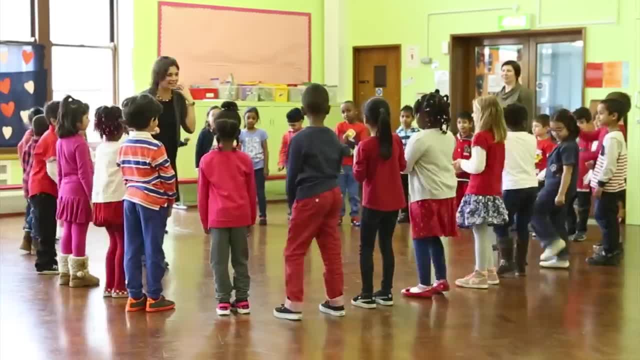 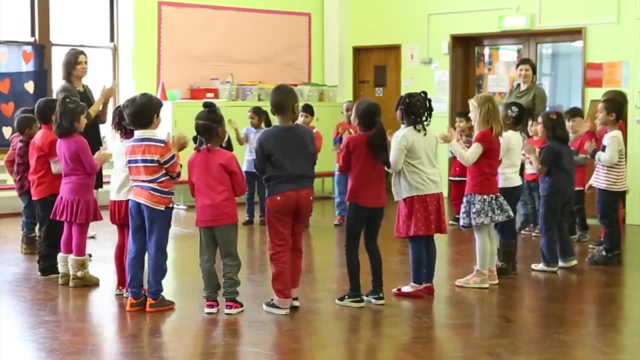 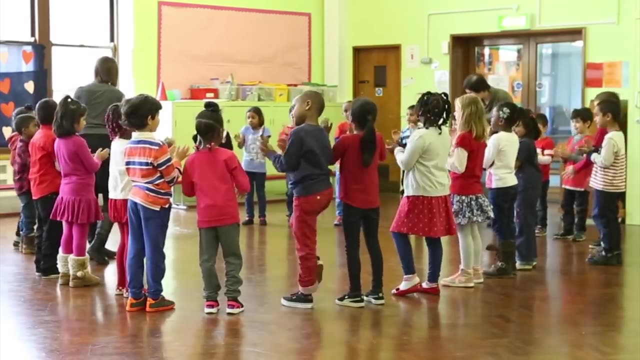 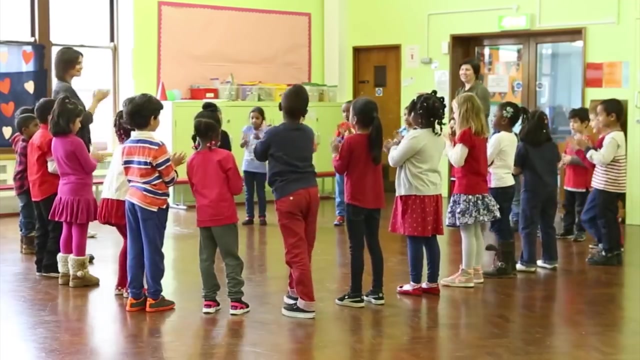 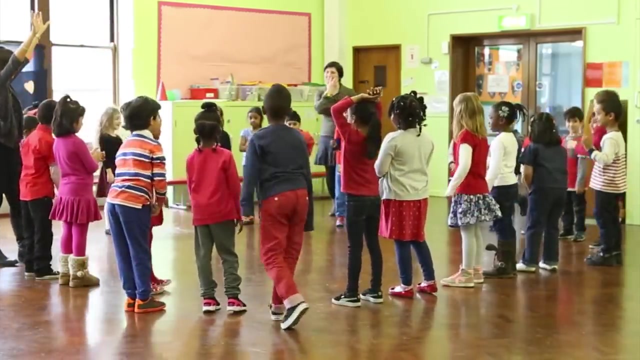 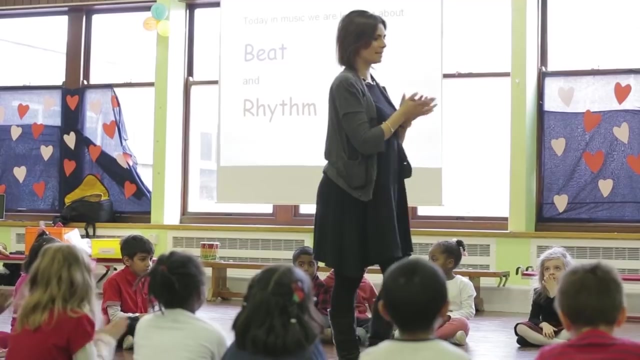 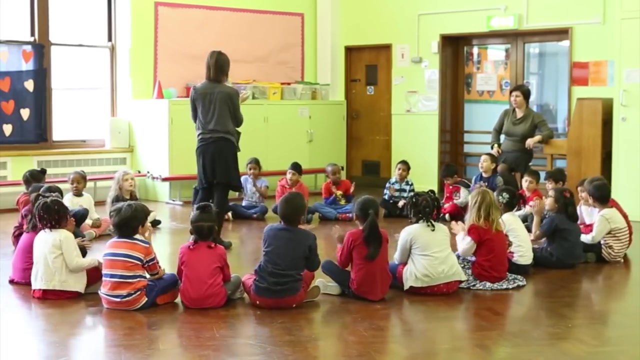 Well done. Now we're gonna do it again, and I really want you to sing even louder this time: Ready, Ready, Fantastic. And freeze This old man. he played one. He played big back on my drum With a knick-knack. paddywhack, give a dog a bone. 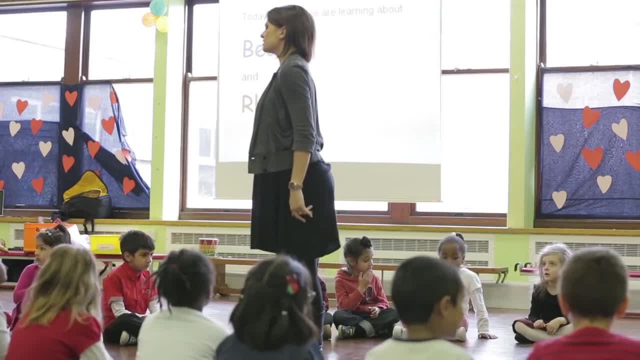 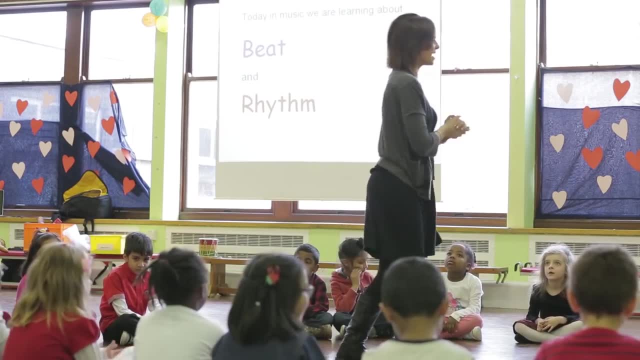 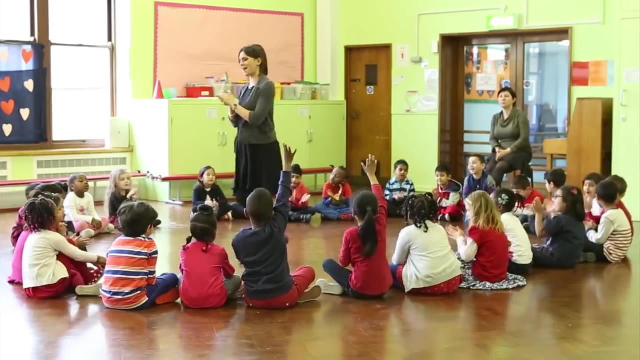 This old man came rolling home. Beat or rhythm, Don't shout out Beat. Well done This old man. he played one. He played one. He played big back on my drum With a knick-knack. paddywhack, give a dog a bone. 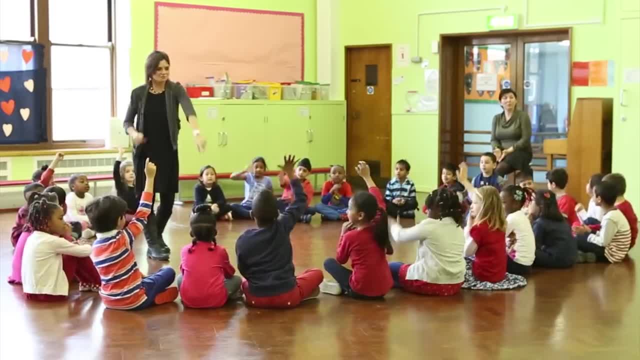 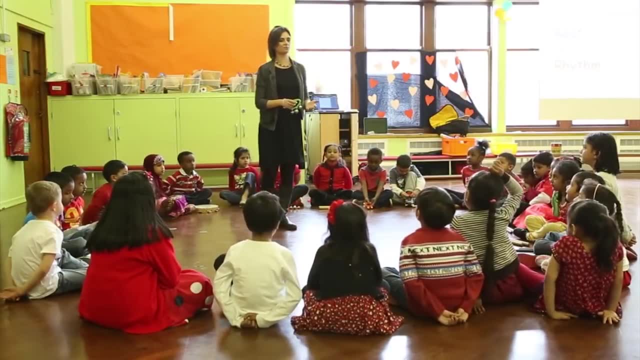 This old man came rolling home: Rhythm, Rhythm. OK, Now show me, you go sitting. Can somebody tell me if I am playing the beat or the rhythm? Listen, Okie-tokie on da. Okie-tokie on da. 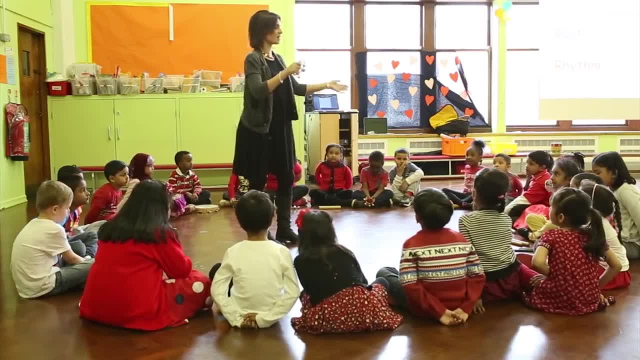 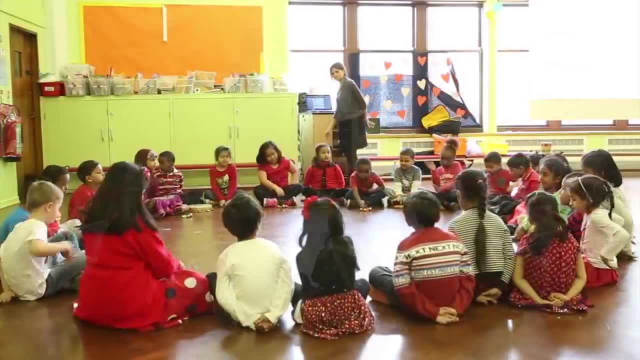 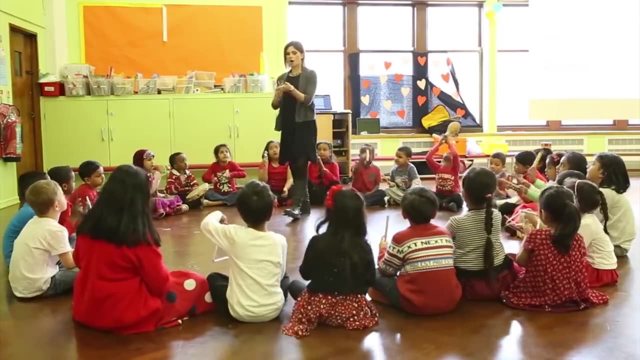 Rhythm. And then we're gonna go Hexacolour, missile warning. It's What is it? Speed, Speed, Get ready. Can I just squeeze through So rhythm Ready? Okie-tokie on da, Okie-tokie on da. 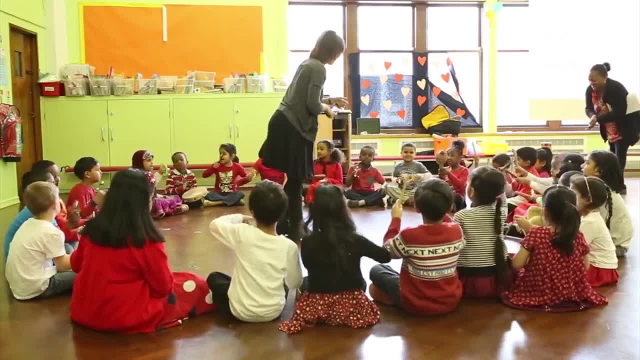 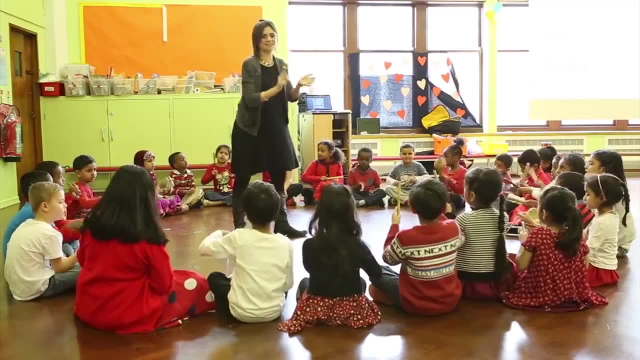 Hey mister, Hey mister. Rhythm: Okie-tokie on da Okie-tokie on da Okie-tokie on da. Hey mister, Hey mister, Hey mister Beat. 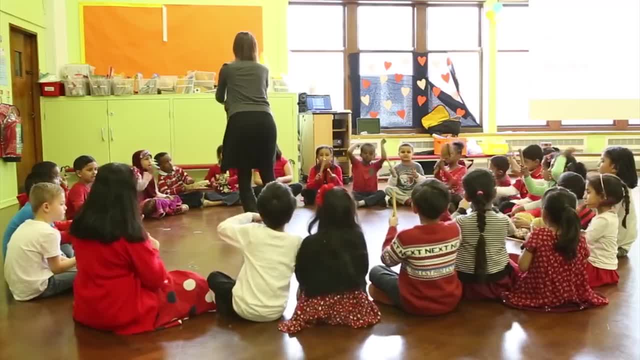 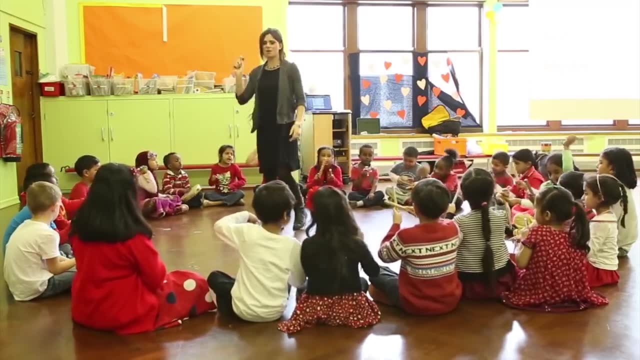 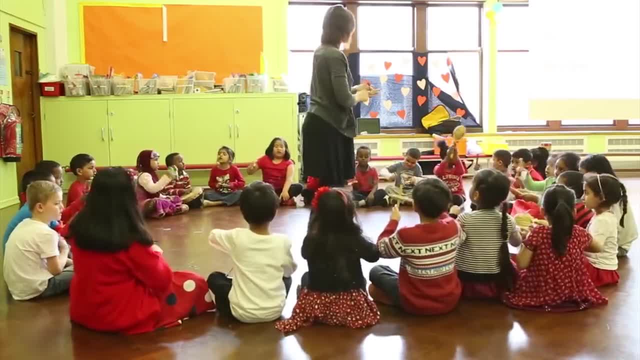 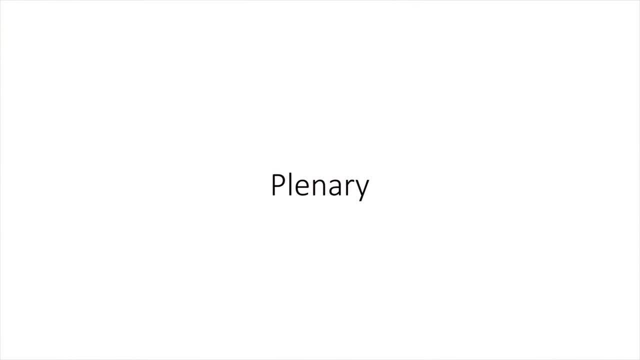 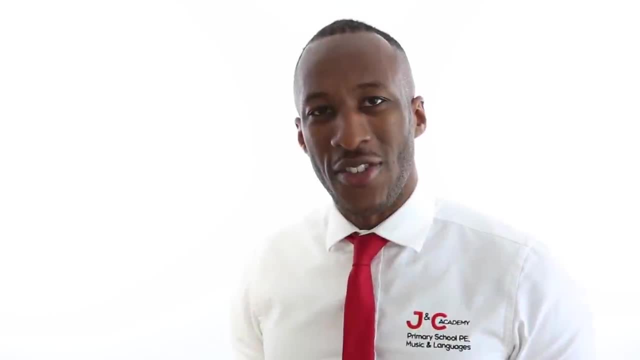 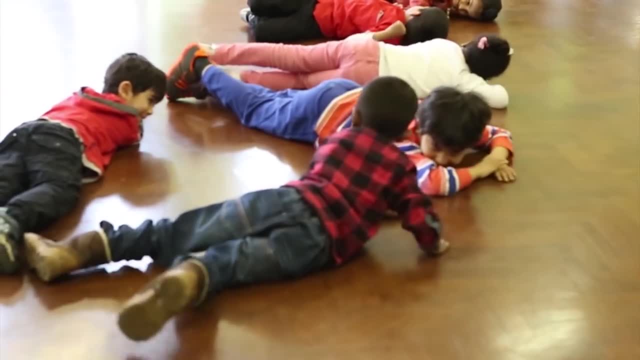 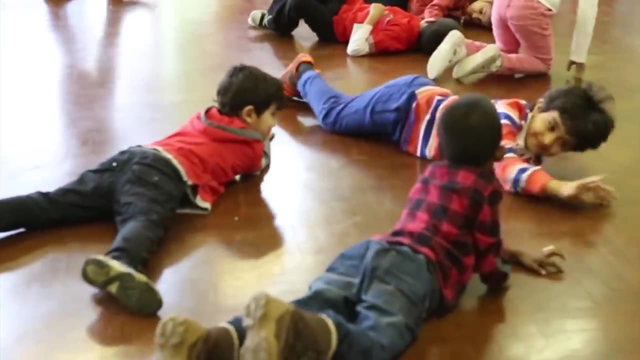 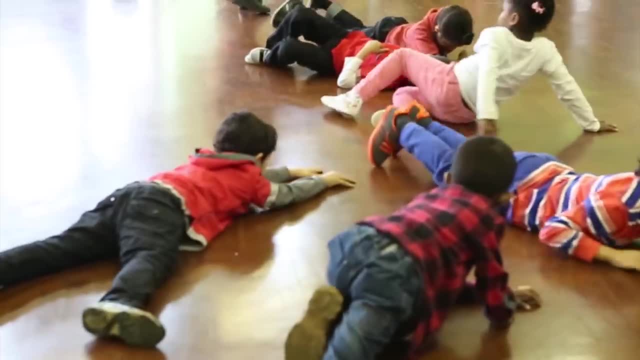 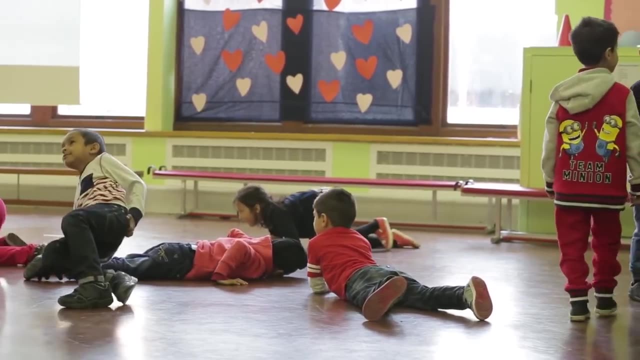 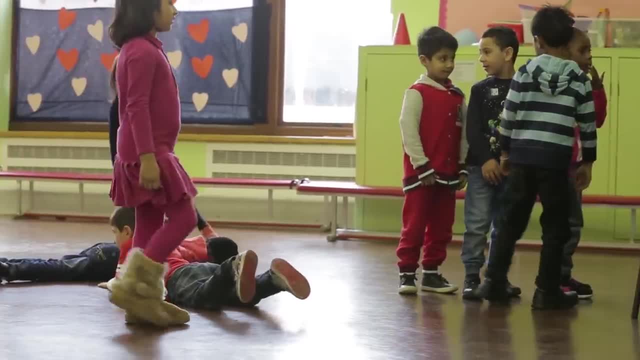